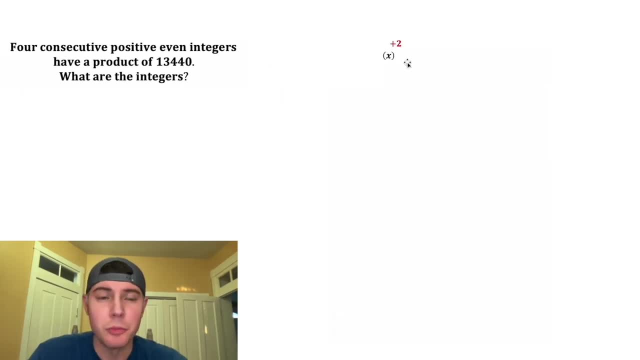 even integer x. So the next even integer will have to be two more than that, So it'd be x plus two. And then we do the same thing to get the next two integers And we need these to multiply to 13,, 440.. Next, if we multiply all these out, it's going to take us a while and it will give us 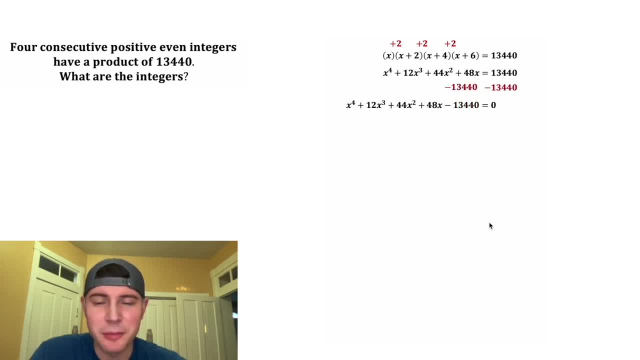 this right here, And then we can subtract 13, 440 from both sides and we get all of this equal to zero. This can be solved, but it'll take quite a bit of work. Let me show you a shortcut. Instead of having the four terms be these, let's have them. be these right here. They're all still. 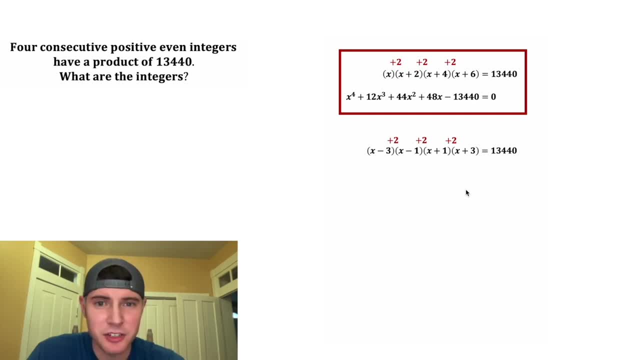 two apart from each other. So these are four consecutive, even integers. They're just expressed a little bit differently, And if we rearrange them like this, then we have a difference of two squares and another difference of two squares. So x plus one times x minus one is just x squared minus one. And then 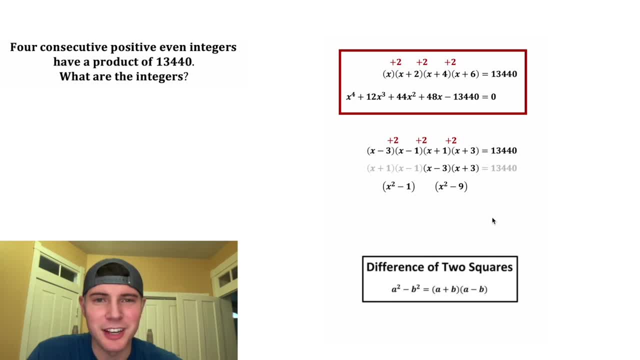 x minus three times x plus three is just x squared minus nine. And then multiplying these out is significantly easier than multiplying this out. x squared times x squared is x to the fourth. x squared times negative nine is negative. nine. x squared Negative one times x squared is negative. 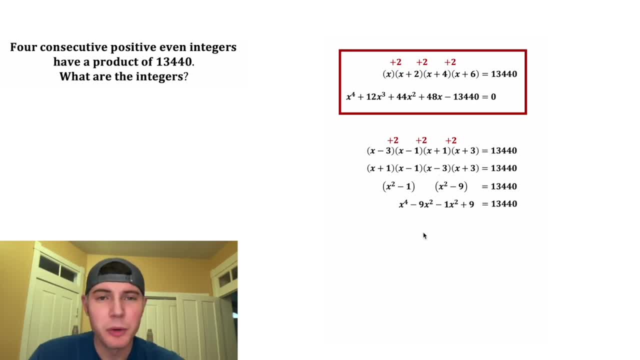 one x squared and negative one times negative nine is positive nine. We can combine like terms. This negative nine x squared minus one x squared will become negative 10 x squared, And then we can subtract 13,, 440 from both sides and we end up with x to the fourth, minus 10 x squared, minus 13,. 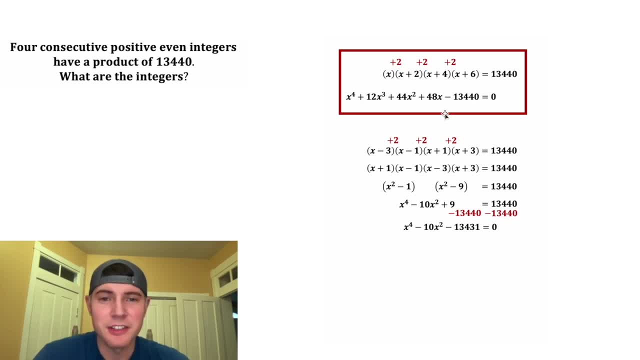 431 equals zero. This is significantly easier than this. We can factor out this left-hand side. We need two numbers that add to negative 10 and multiply to negative 13, 431.. This will take a little bit of trial and error, but that ends up being negative 121 and positive. 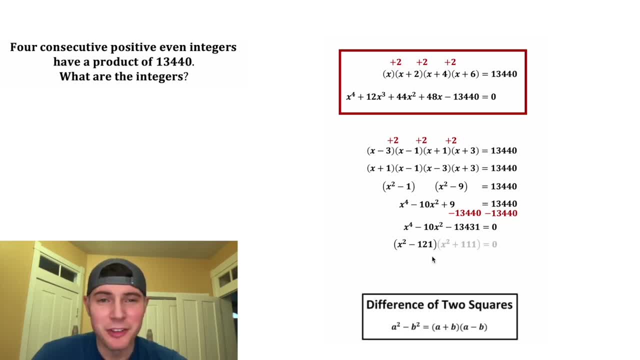 111.. And then x squared minus 121 is another difference of two squares. That gives us x minus 11 times x plus 11.. And then we can just copy down the rest of this stuff And now that we have this factored, we can solve for each of these, For x squared plus 11 equals zero. we can subtract 11.